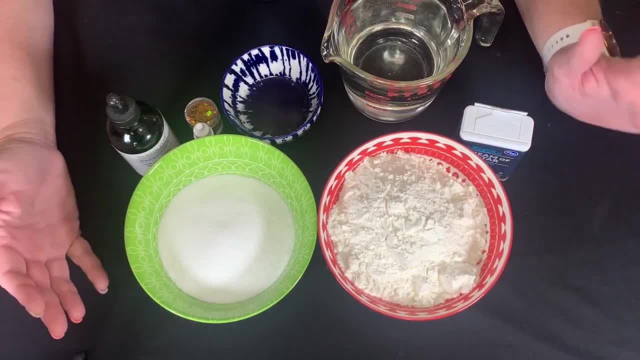 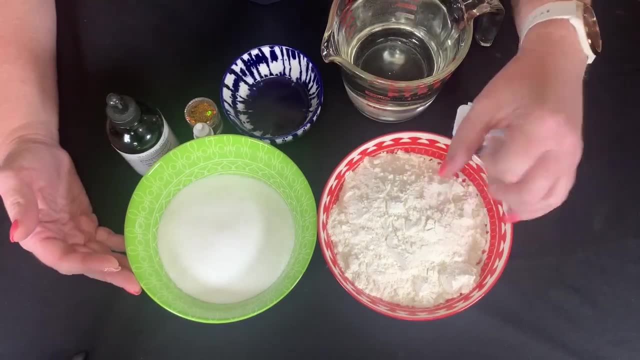 customizable or customization ideas. So something for gosh just about every week of the year, every week of the school year. certainly, Today we're going to be making. today we're going to be making some money-based Play-Doh, or some money Play-Doh, because we're 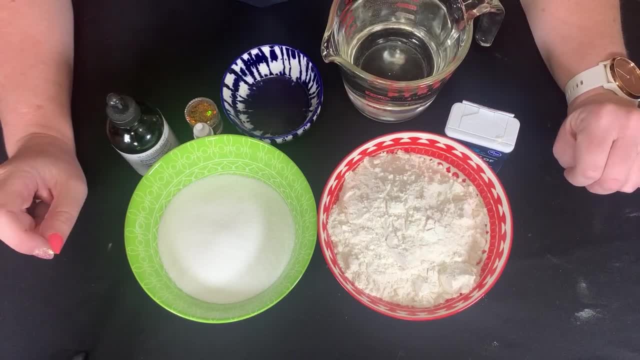 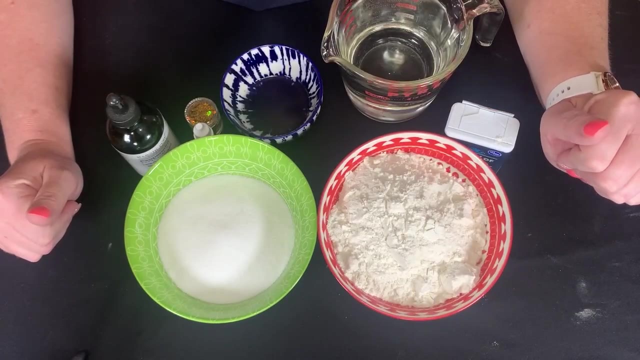 still kind of working about. on Alexander, We're talking about Alexander, who used to be rich last Sunday and his money that disappeared. So we are going to make green Play-Doh with kind of a peppermint scent. Let's talk about what our ingredients are. here We have two cups of flour. 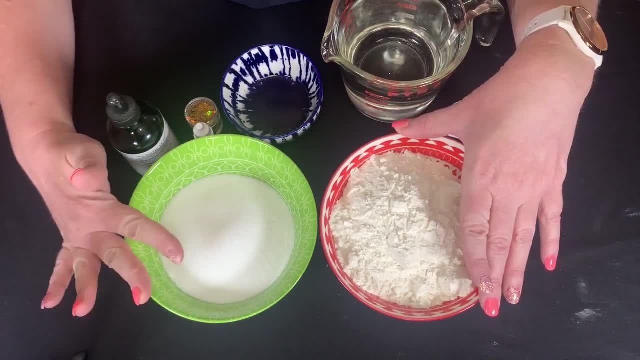 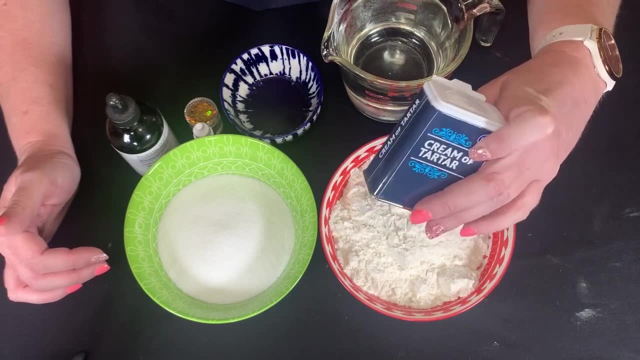 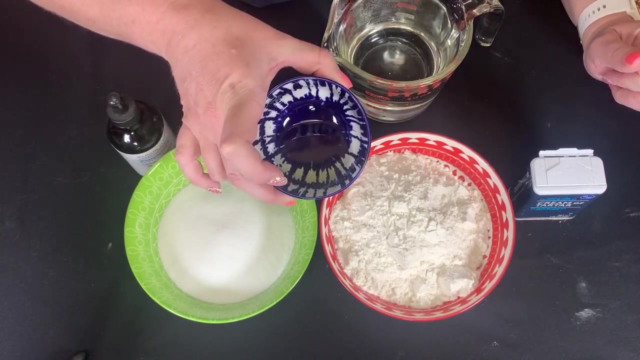 just regular all-purpose flour, nothing special needed One cup of salt. We're going to put in two tablespoons cream of tartar and you can just get the this in the baking aisle- Pretty common. We also have two tablespoons of oil and I just used. 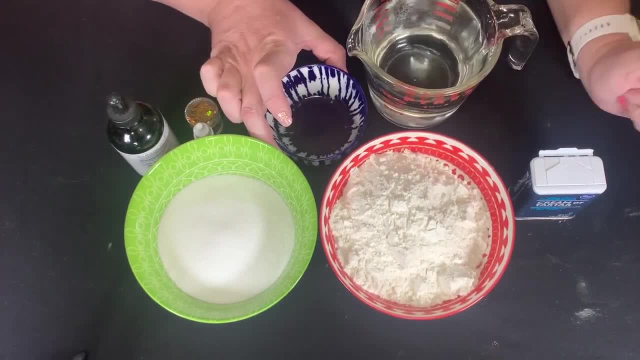 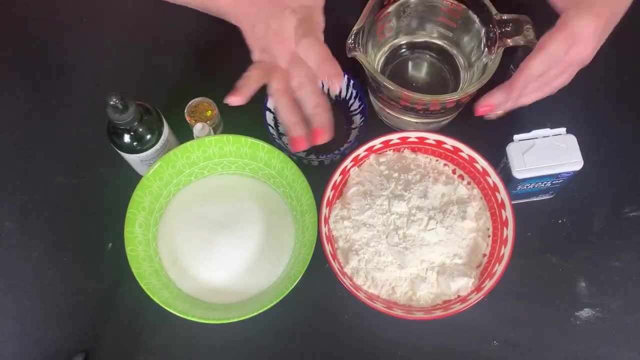 canola oil. You can also use vegetable oil, You can use olive oil, but it gives it a little bit of a scent, a little bit of an olive oily scent. And then two cups of boiling water, And that's what you need for just the base recipe, Every Play-Doh recipe, or every Play-Doh recipe that I. 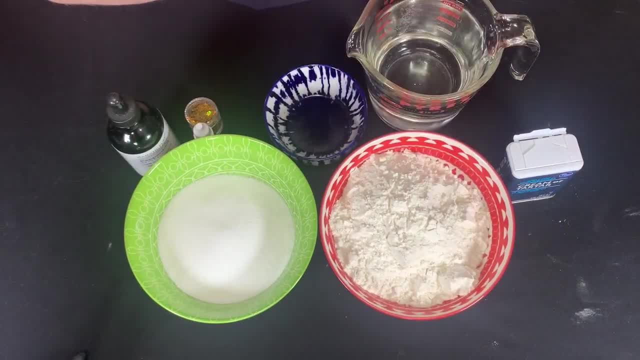 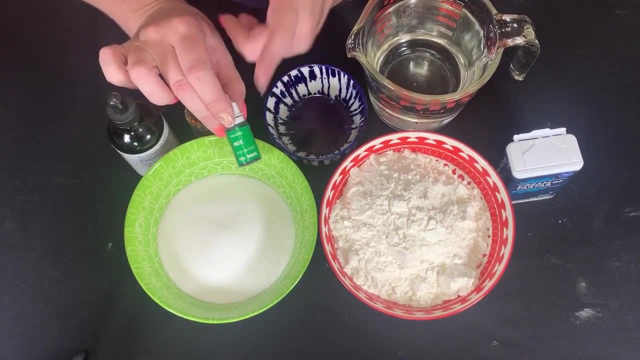 have involves these ingredients and then you customize from there. For today's customization, we're going to put in some green food coloring. I like to use green because we're using- we're talking about money. This is liquid food coloring. You can also use gel food coloring or you can use tempera paint if you want. I just know that. 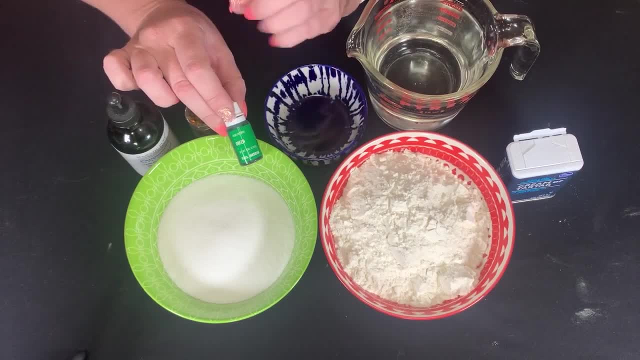 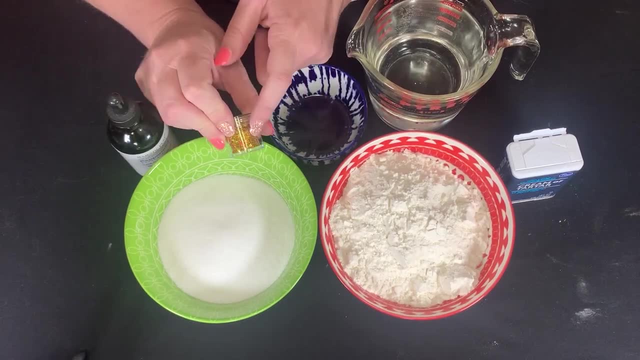 when I use the food coloring, it's definitely non-toxic If it gets eaten. basically anything on this table is edible, Minus the glitter that we're going to add to it. I'm not a huge fan of glitter and I try to avoid it. And I'm not a huge fan of glitter and I try to avoid it. 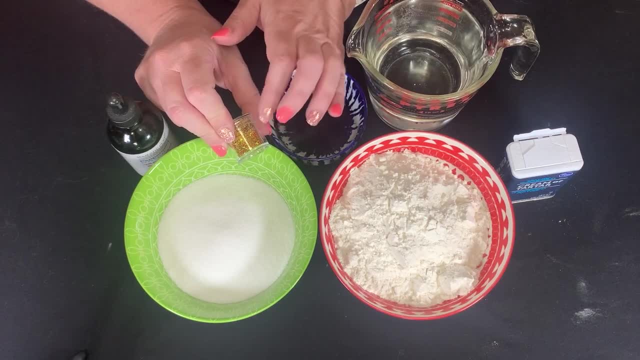 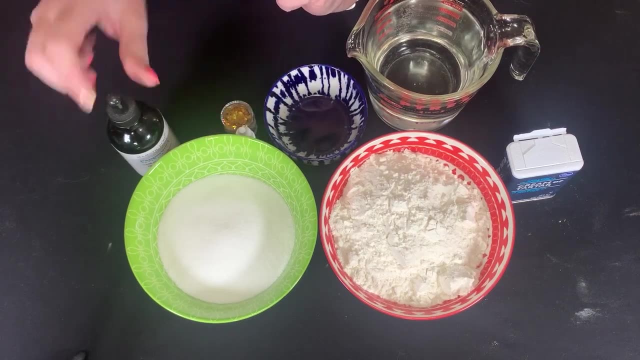 My craft projects, because I find it gets everywhere. but I'm willing to take the risk for this Play-Doh, just to add a little bit of sparkle to it. And then, finally, I'm going to add some peppermint essential oil to it just to give it a scent. 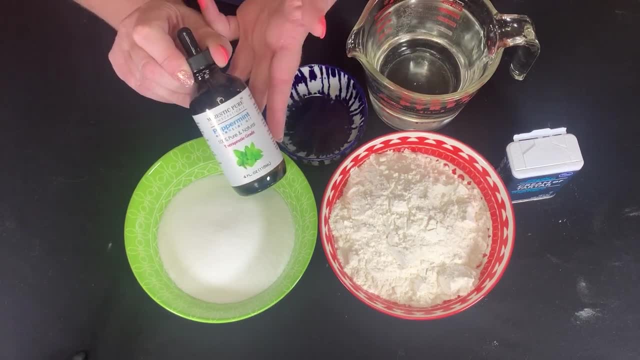 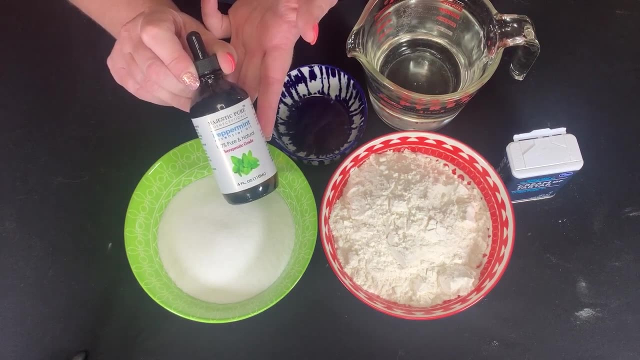 This is kind of a less expensive essential oil. I'm certainly not going to use a super expensive or super high quality essential oil on it because we're not using it therapeutically. We're really just using it to give some scent and we're going to use it to engage another. 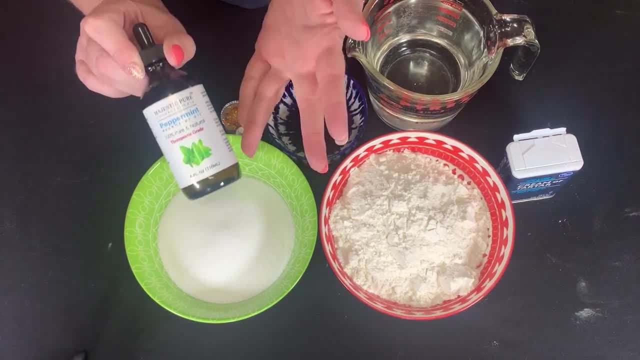 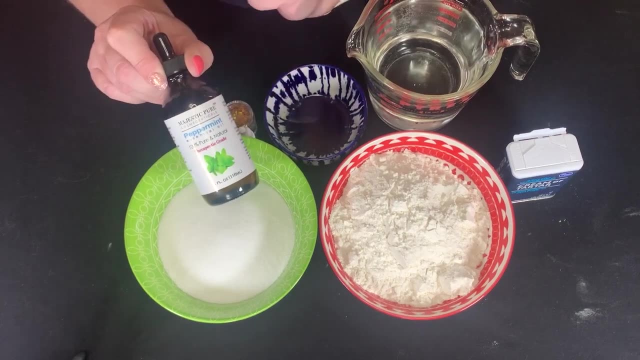 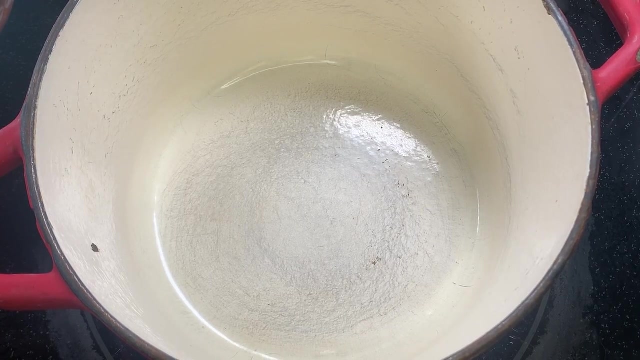 sense. So we're going to have the sense of touch, sense of scent, sense of sight. Those are three that we're going to use right there, So that scent adds to that. All right, let's get started. Let's get started on our Play-Doh. The first thing we're going to do is mix our dry ingredients. 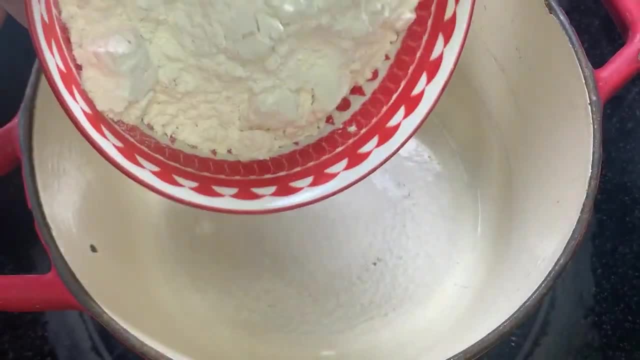 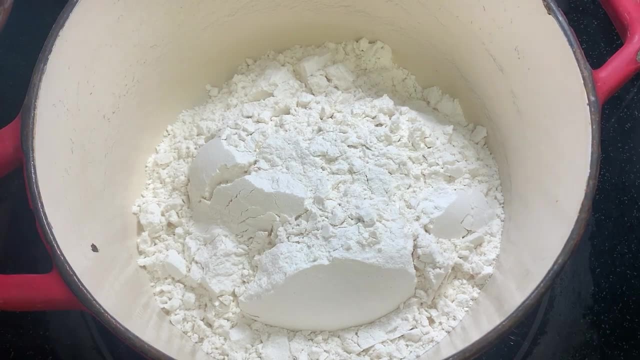 together. So we're going to go ahead and put in that two cups of flour- Again, that's just plain old. all-purpose flour. We're going to add that to our Play-Doh. So we're going to add that to our flour. We're going to mix in. we're going to add in a cup of salt. Same thing, just plain old. 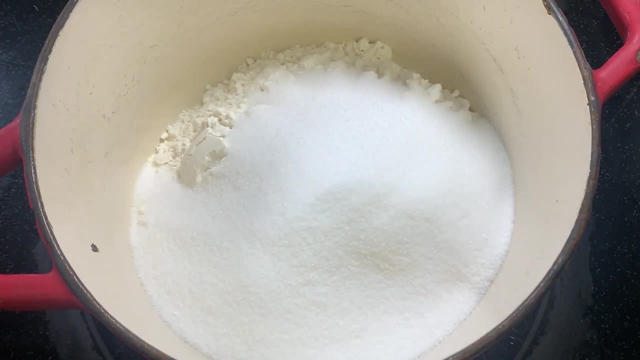 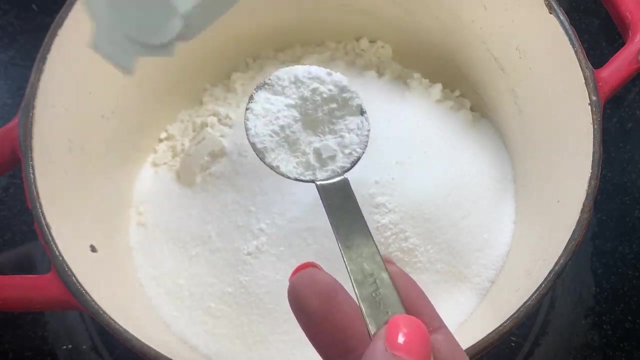 regular salt. The one with the little girl on the front cover is fine. Then we're going to put in two tablespoons of cream of tartar. And, guys, this isn't like we're not doing brain surgery here, so it can be. 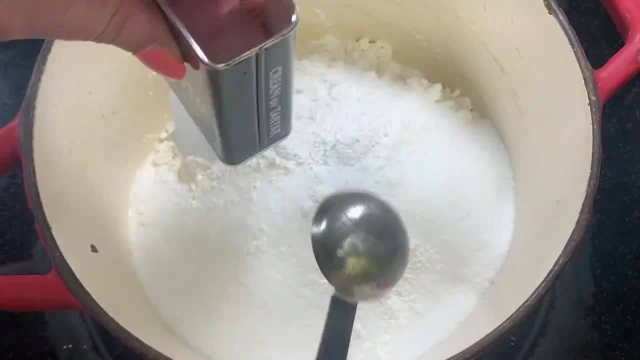 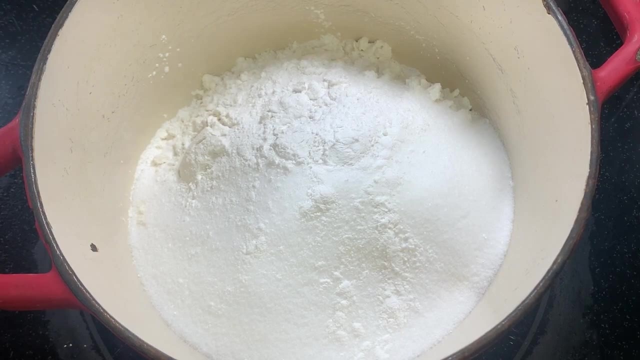 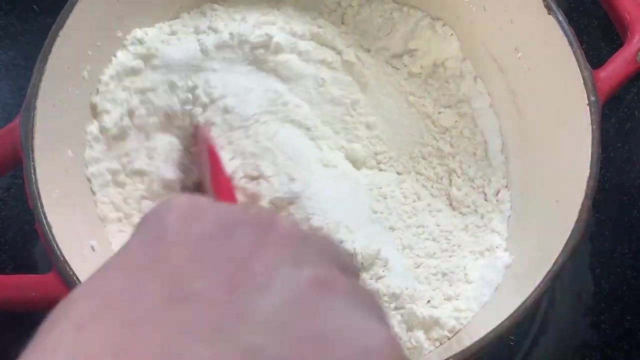 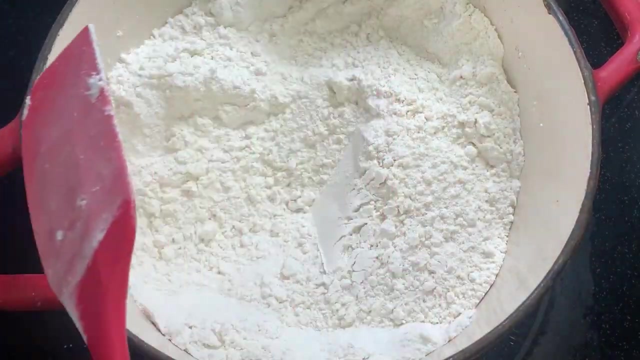 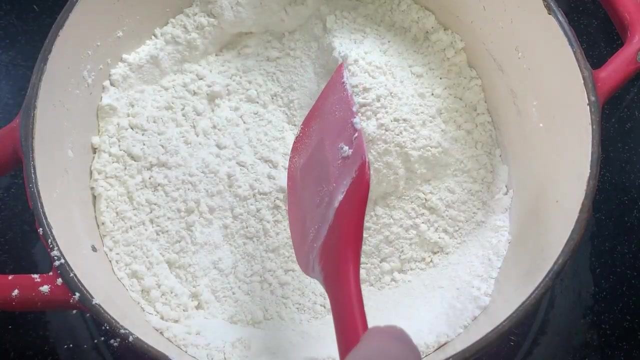 You can do roughly that much. Okay, we're going to mix those together, Get our dry ingredients pretty homogenous, And then we're going to turn the oven on. We're going to go medium heat And we're going to gradually mix in our boiling water. You can see the steam rising off of that. 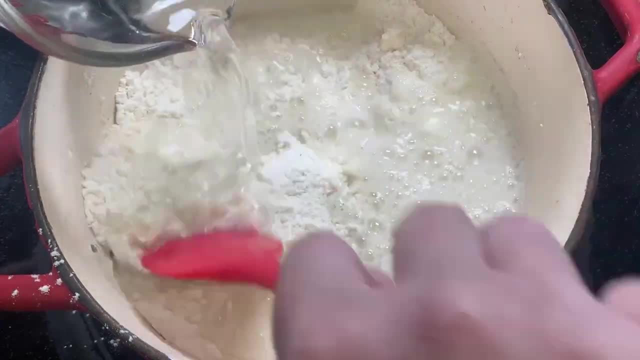 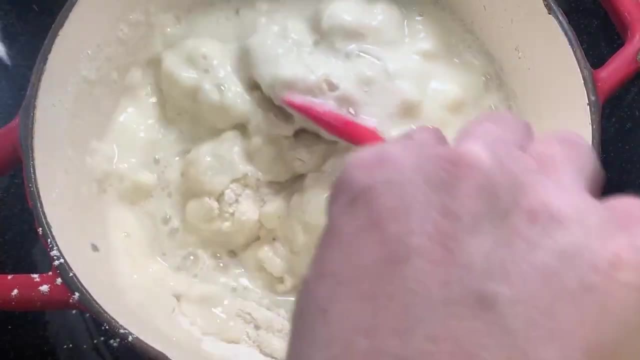 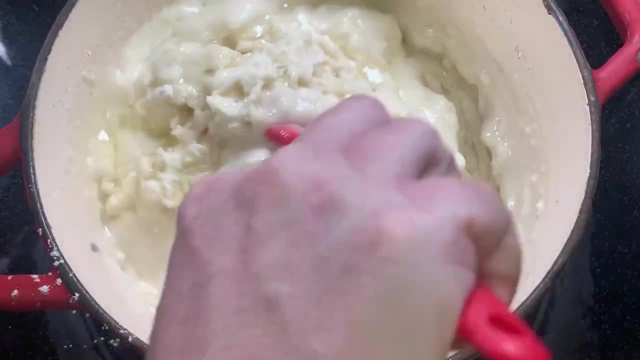 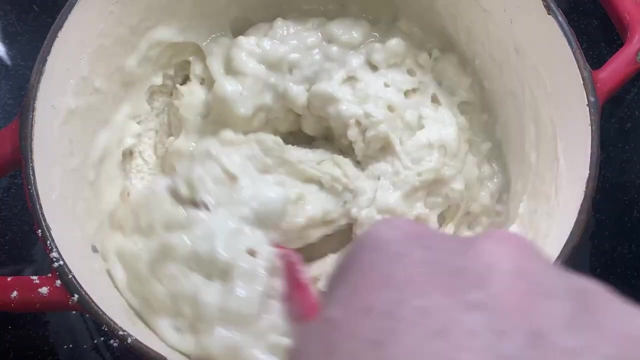 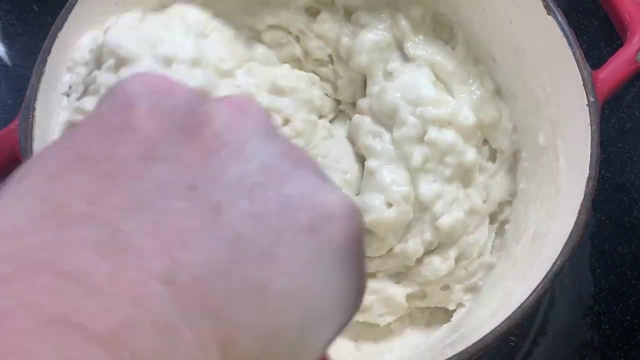 maybe It is. get that stuff boiling. Keep mixing that And add in the oil. Give that a good mix up. You can see how there are some chunks in there. We want to mix those all out And there's some spots where it's still dry. Get that nice and smooth. 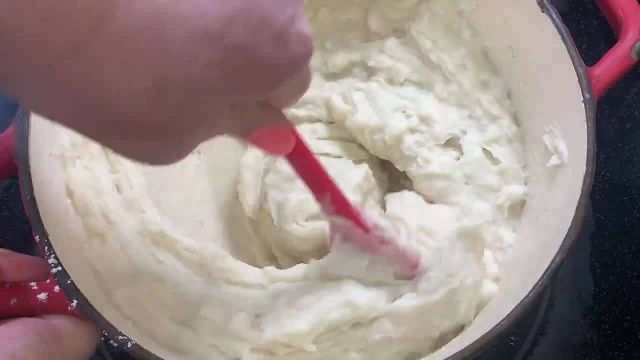 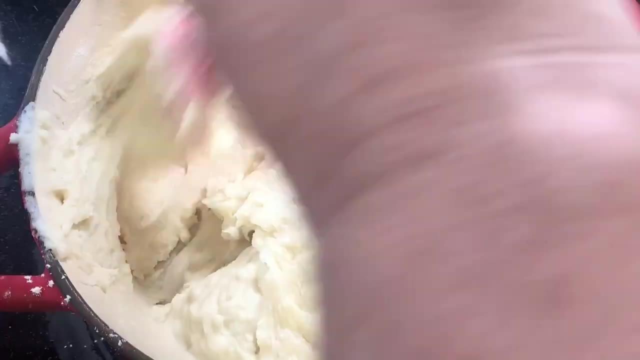 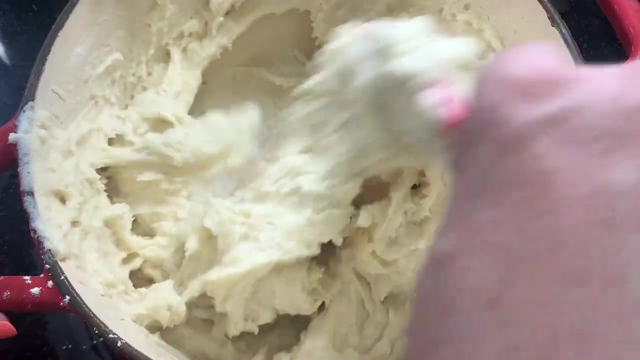 What you can do if yours is really chunky is get a whisk when you're first starting to mix it And whisk it all together. Now see how this is kind of forming up into a paste. It's going to form into a ball. 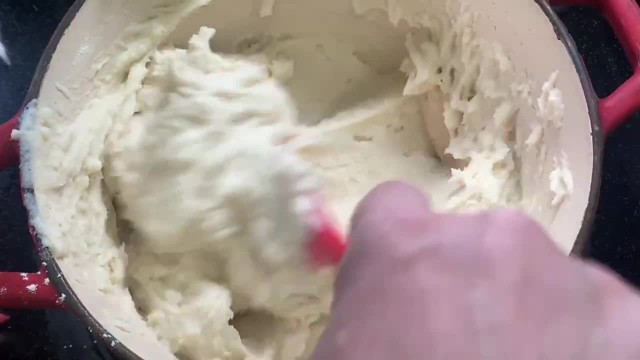 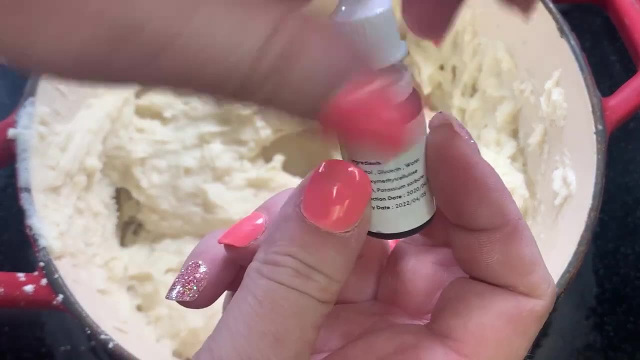 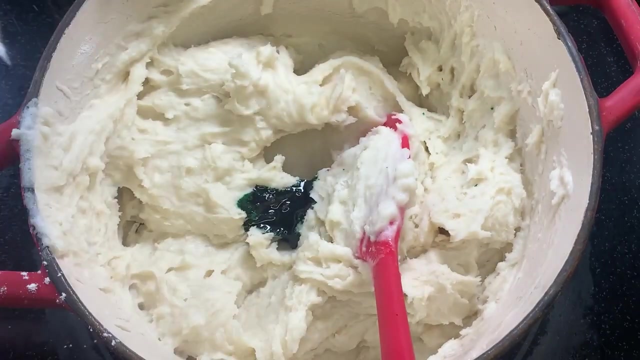 And that's when we'll pull it off. While we're waiting for this to form into a ball, let's add our mix-ins in. So again, here's that green food coloring. Mine is drops. You can also use gel, And I'm going to put a pretty decent amount in there. 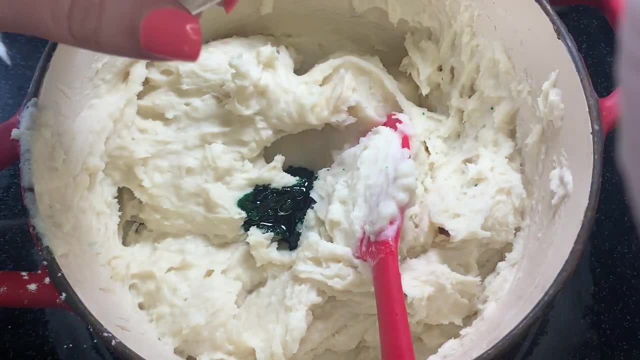 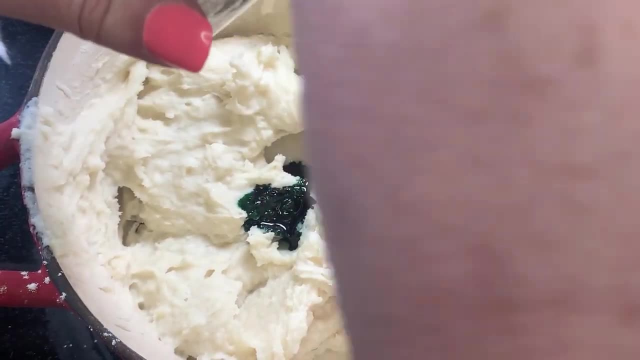 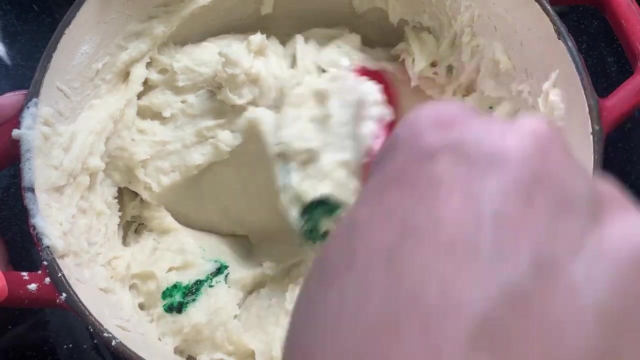 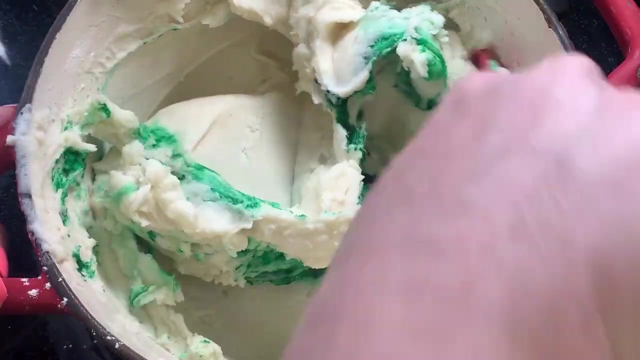 I am also going to put in one dropper of peppermint, And you know what? Just for the heck of it, let's put in a second dropper Again, it's not precision crafting. See how already, just in the amount of time it took me to mix in or to add in those customizers. 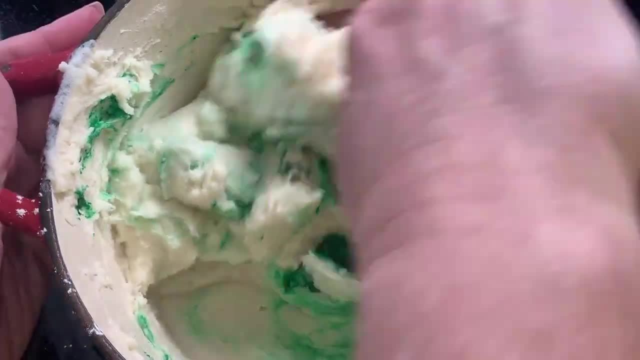 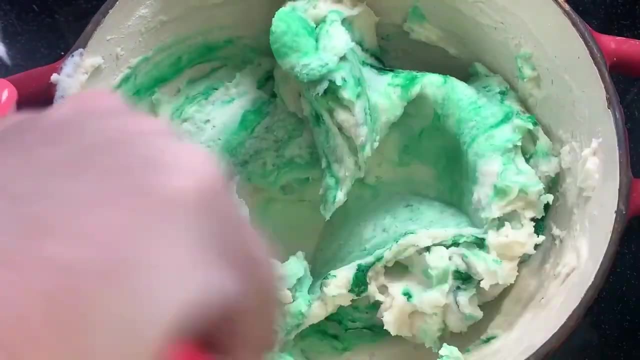 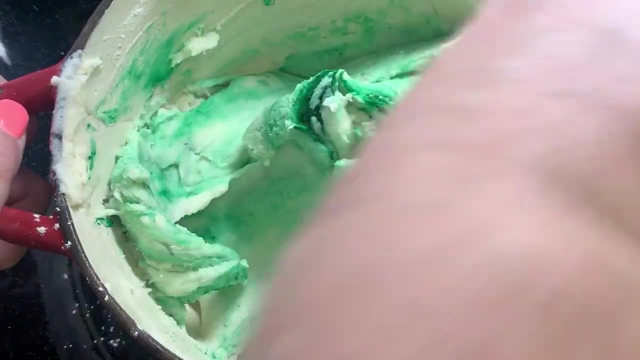 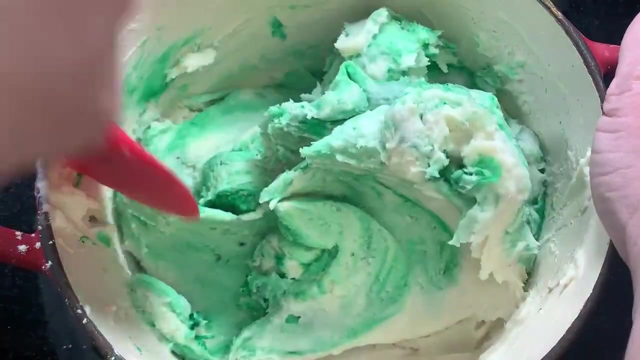 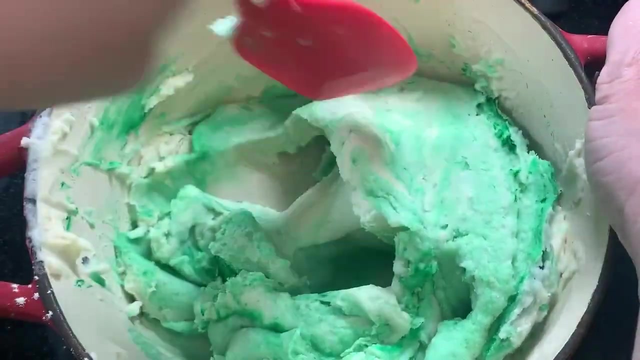 it's already getting More and more solid. Did you know that Play-Doh was originally invented in the 30s as a wallpaper cleaner? The guy who invented it envisioned that housewives would slide Play-Doh all over their wallpaper and clean it up, And then teachers found the substance and started using it. 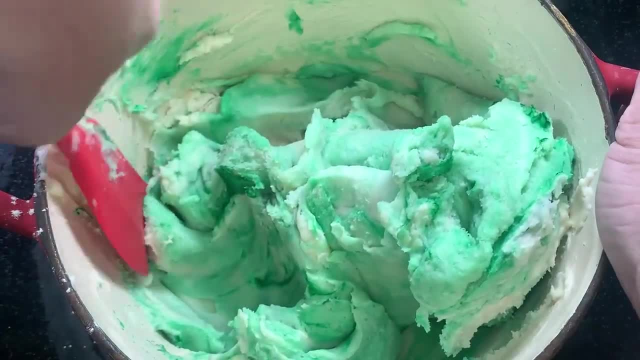 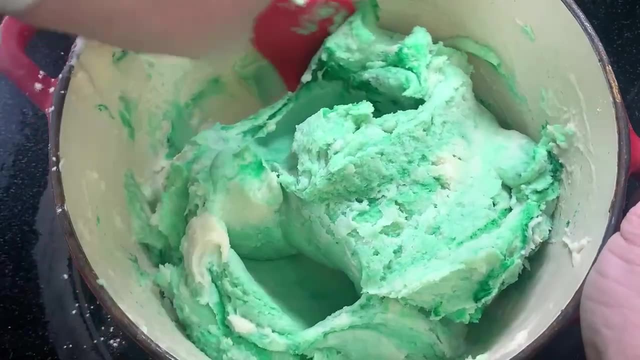 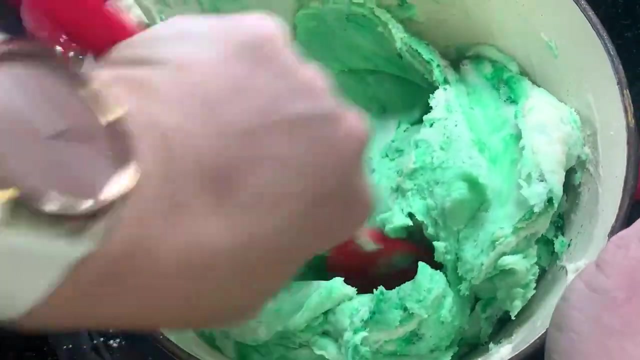 As a sculpting method for their kids. So look, teachers change in the world, Introducing Play-Doh to us as a toy. All right, see how that's really coming together. And the color is pretty kind of variegated, not super smooth. That's okay, because we're going to need this And when we 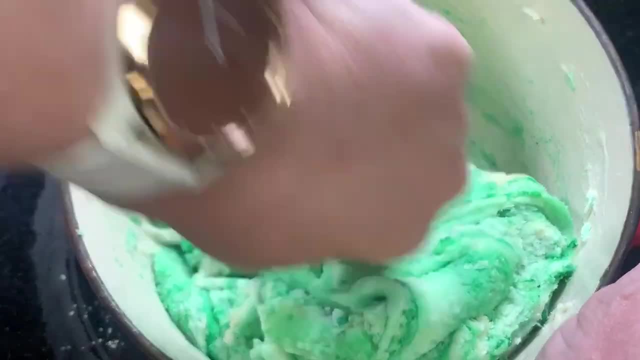 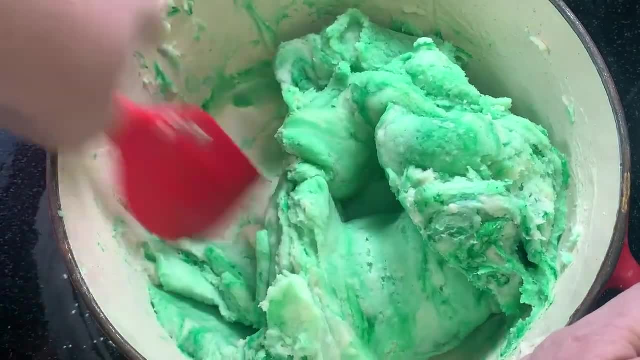 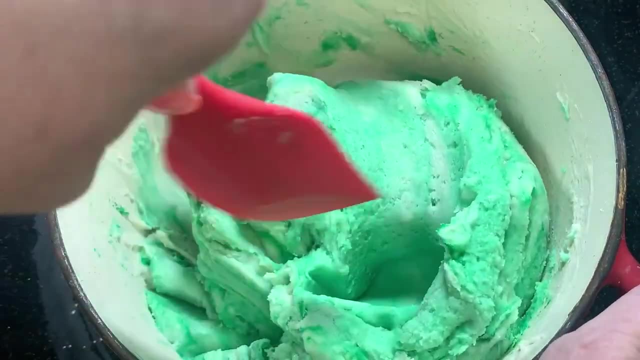 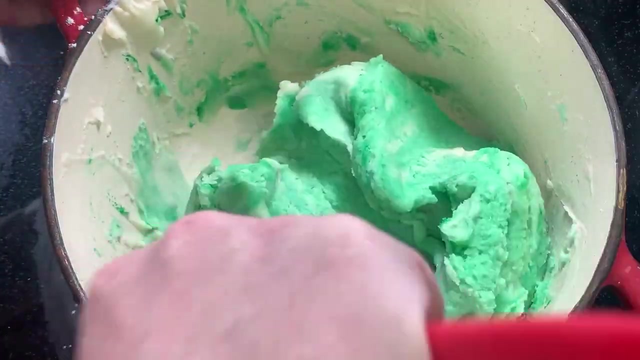 You obviously can't smell this, but holy peppermint smell. Now I know I haven't put the glitter in yet. I'm going to put the glitter in when we need it. This is exactly the consistency we're looking for when we stop cooking it. So we're going to take that off the heat and let it sit. We're going. 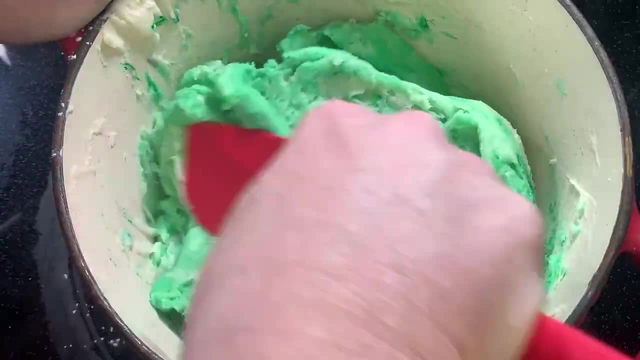 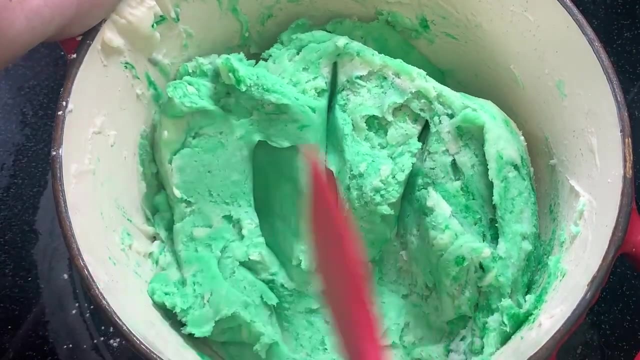 to let it sit for at least a half an hour. Something about this mixture really traps heat, And even when you think it's cool to the touch, there are little hot pockets in there And you can burn the heck out of yourself. Ask me, 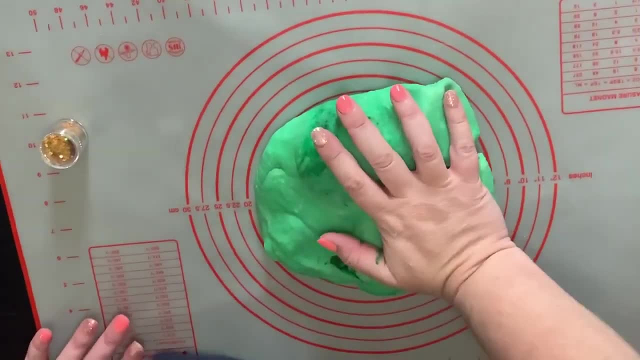 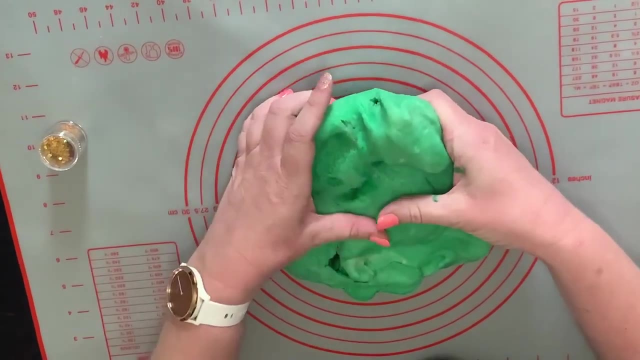 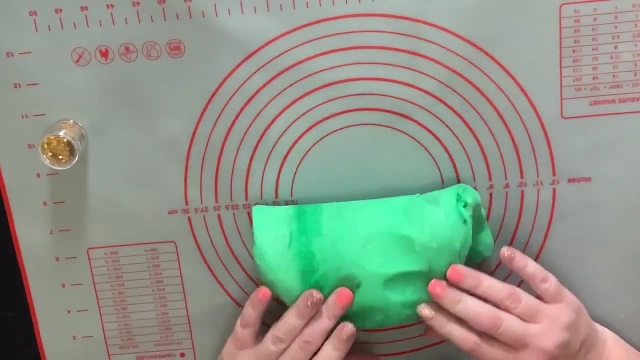 How I know. All right, So we waited our time. Play-Doh is still warm, but it's not like going to burn me, which again it gets some hot pockets in there for sure, And you can see we still have some streaks of green. I don't see any, but there can be just like a little. 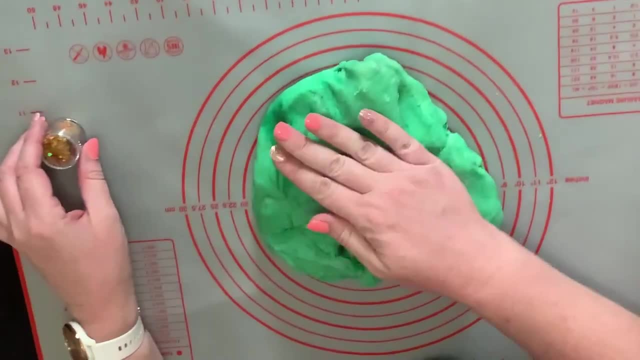 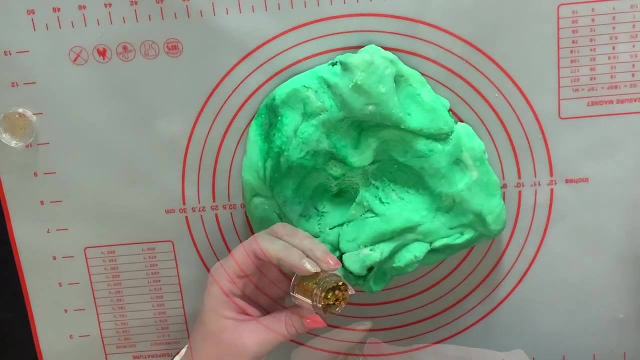 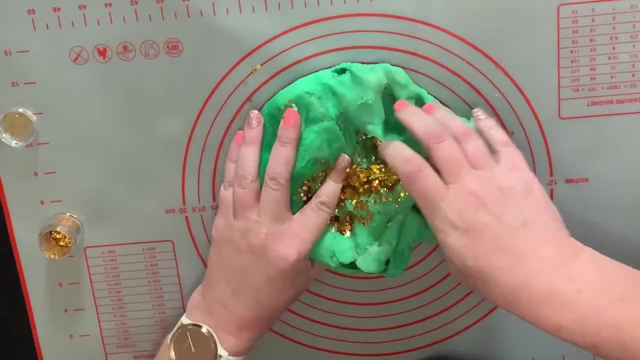 cream color there, So we just need to need it a little bit more. We're also going to mix in our glitter, So I just have some gold glitter just to give it a little bit of shine. I'm going to put in a decent chunk Scrooge McDuck's coins in there, huh. 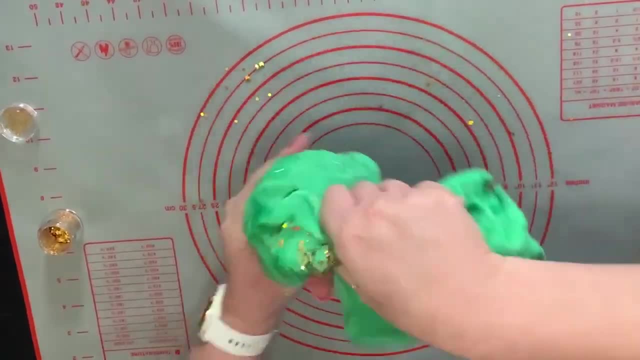 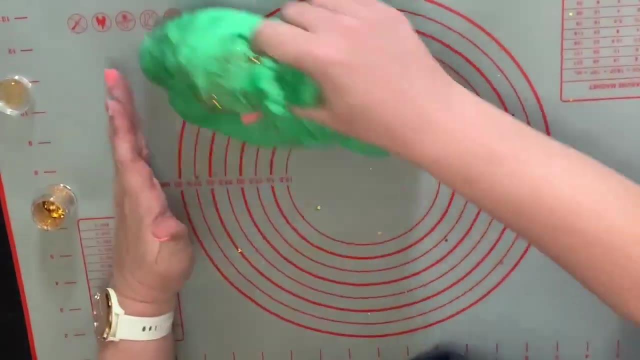 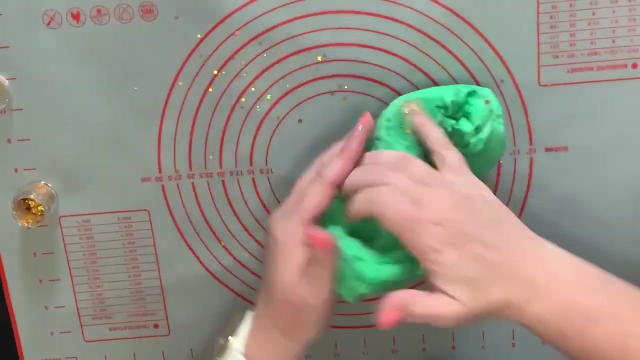 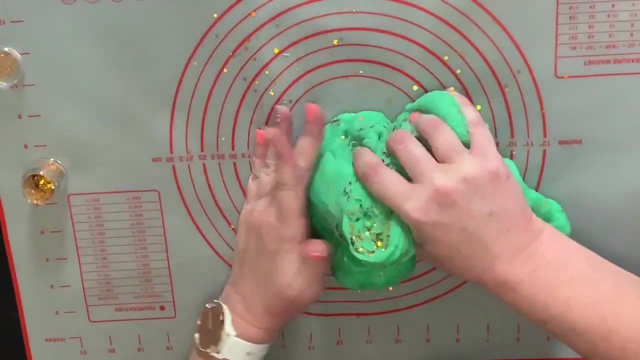 And we're just going to get in and knead it and just get it all so that it's a consistent pick up, that extra glitter, so that it's a consistent color, consistent texture, which the texture should be pretty consistent Anyway, but get that glitter kind of spread through there. You can see I have glitter.